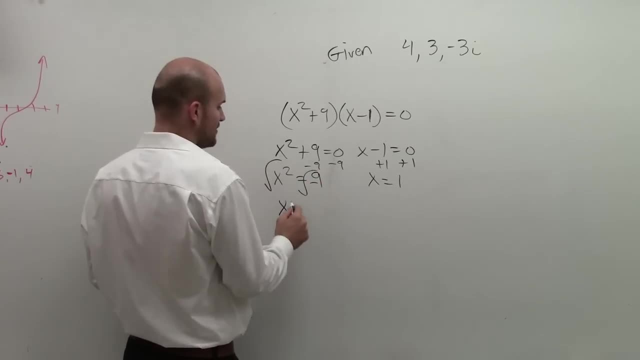 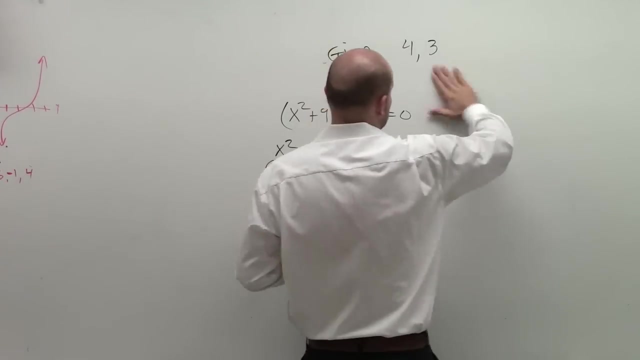 you'd have x squared equals negative 9. Then you square root And remember we always did x equals square root. We always did plus or minus. So that's why- because a lot of times in a test I'm just going to: no, I can't do that- 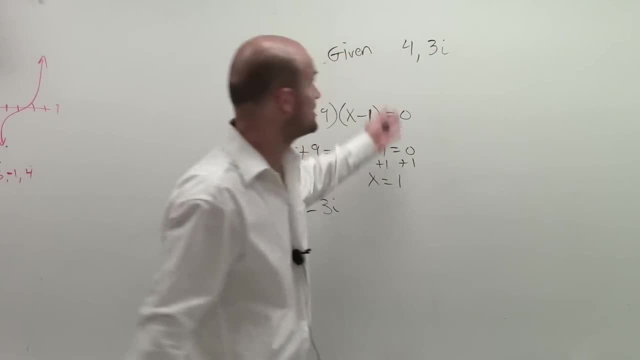 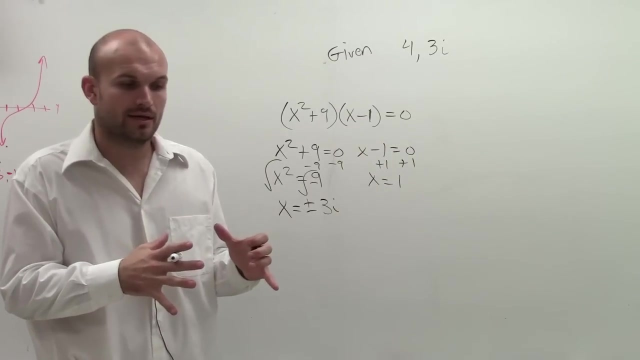 I would say 3i And make sure that's my answer. Yeah, I'd give you 4 comma 3i. Well, remember, if you're given one complex number as a, if you're given one imaginary number as a root, 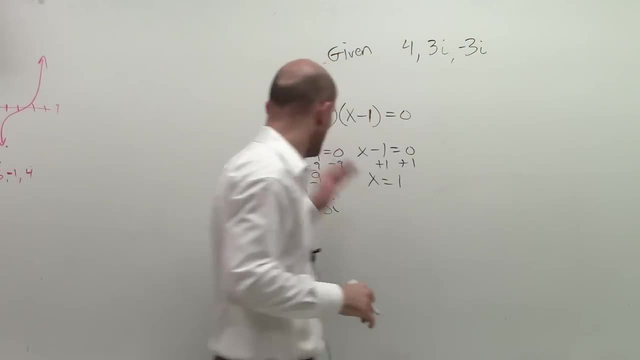 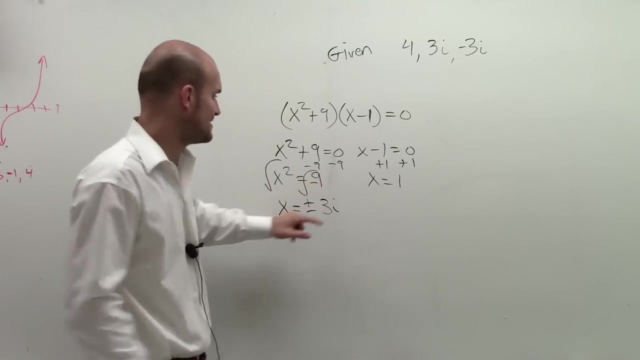 you have to include the opposite value Because, remember, when we take the square root to find the 0, it's always going to be plus or minus. So, notice, I'm going to have both of these be my zeros, So I'm going to have both of these be my zeros, Meaning I can write both of these as factors. 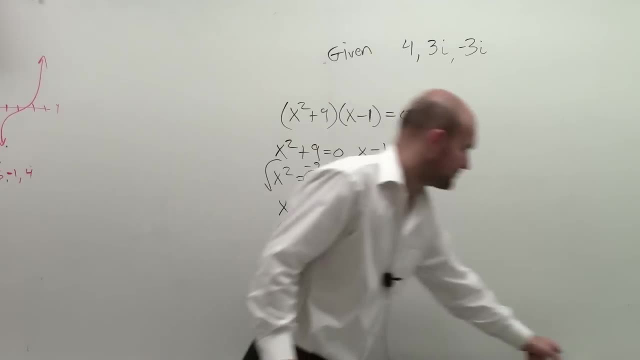 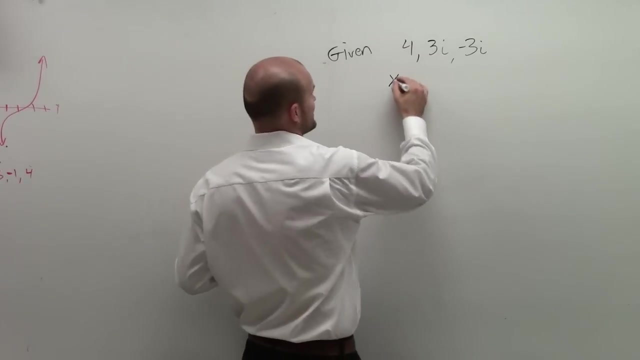 like this: All right. So what we're going to do is we're going to take our zeros And we're going to write it as a series of factors. So to do that, I say x minus 4 times, x plus 3i times. 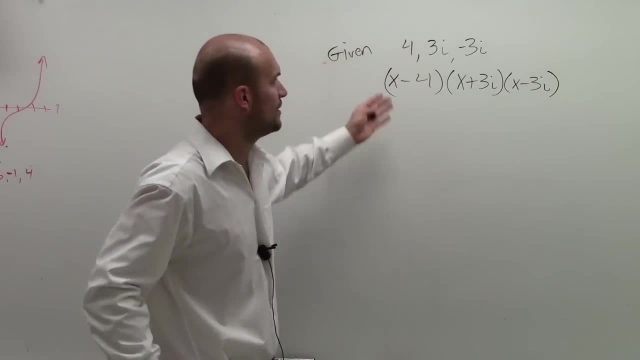 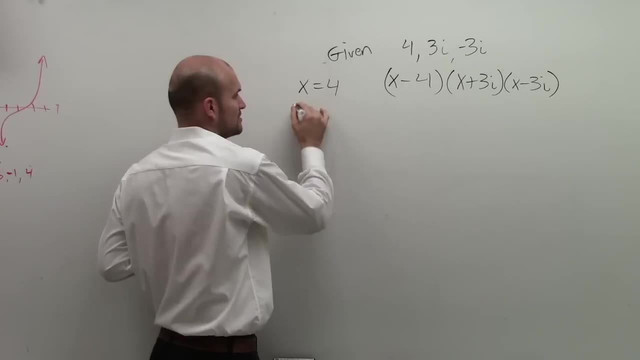 x minus 3i, All right. And if you want to do that, if you want to go from, how did I get x minus 4?? Well, remember, if that's my 0, that means the x intercept equals 4.. So 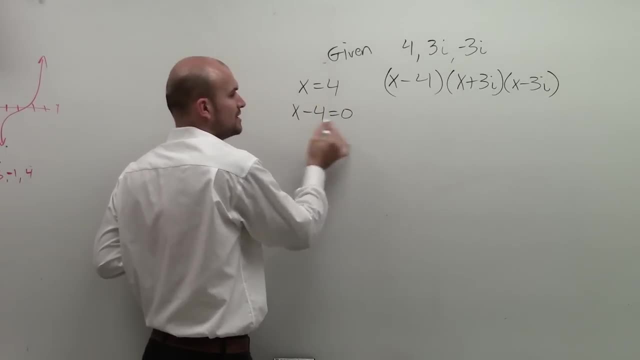 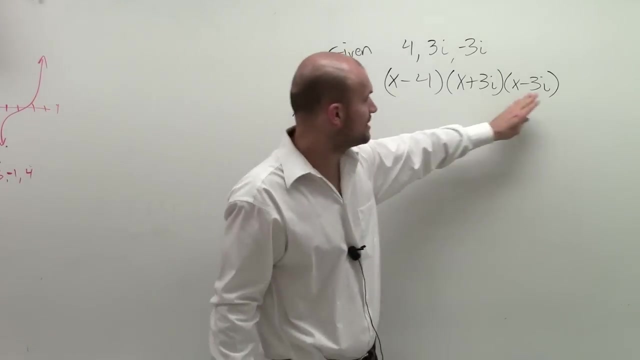 I set that equal to 0. So I subtract the 4 on the other side, So I get x minus 4, meaning that's my factor. OK, So now what I'm going to do is I'm going to multiply. Well, I'm going to multiply this. 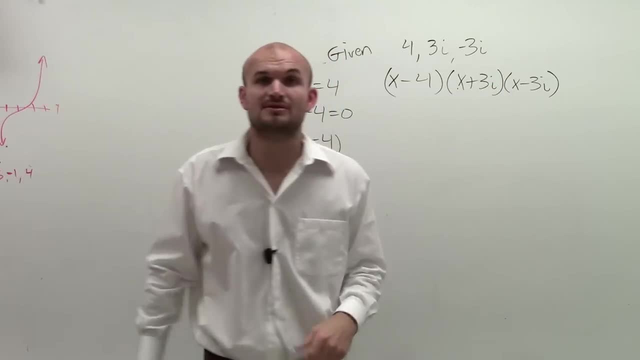 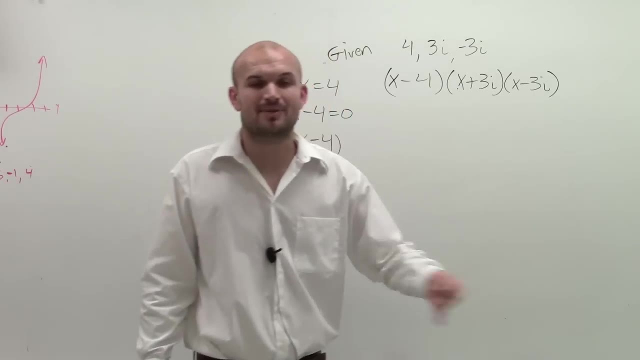 first, because what I notice is my first two terms are the same. Last two terms are the same. That's the difference of two squares. We've got to remember the difference of two squares because it helps us multiply so much quicker And we see this that we don't have. 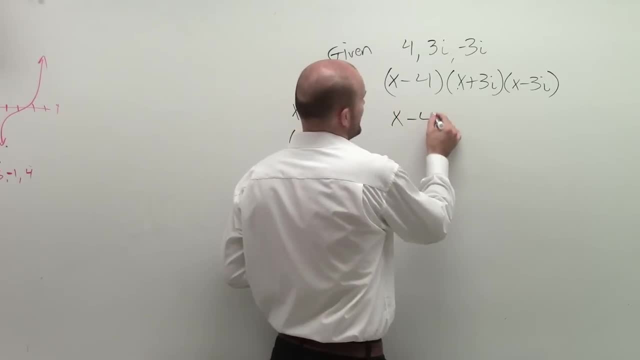 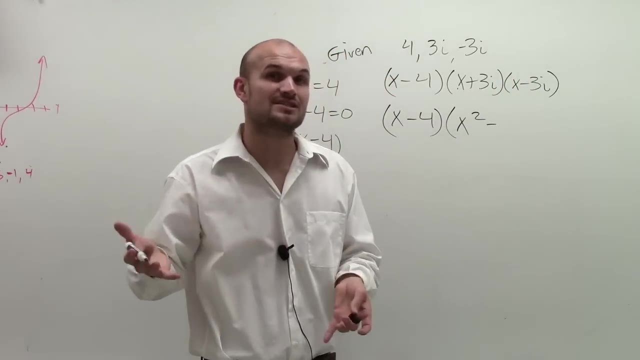 to even follow the FOIL and all that kind of stuff. We can easily just rewrite this Now as x squared minus 3 times negative 3 is negative 9.. But then times i squared- i squared is negative 1.. Negative 1 times negative 9 is now going to give me positive. 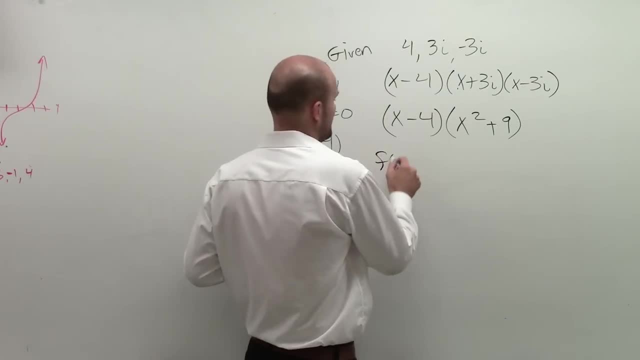 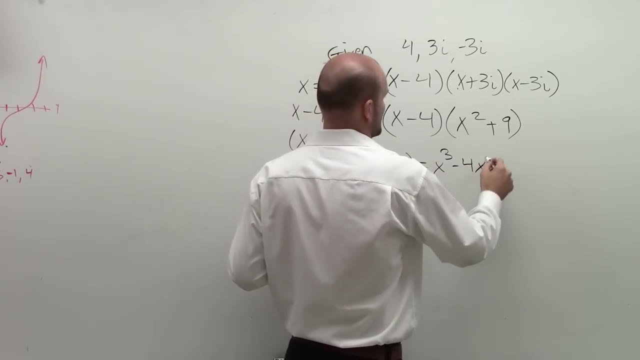 9. Now I need to multiply these two So I have f of x equals these two binomials multiplied, So I get x cubed minus 4x squared, plus 9x minus 36.. So there you go, ladies and gentlemen. 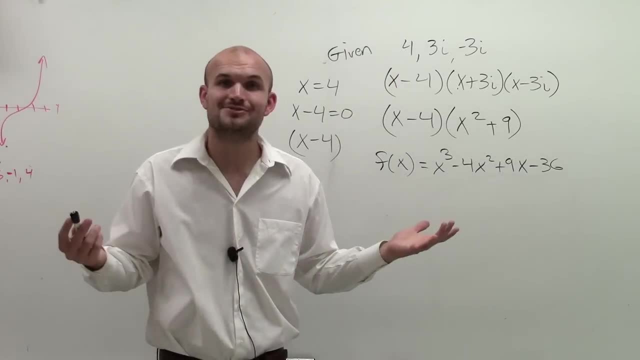 That's how you multiply when you have x squared minus 4x squared. So you have given zeros to find your polynomial Thanks.